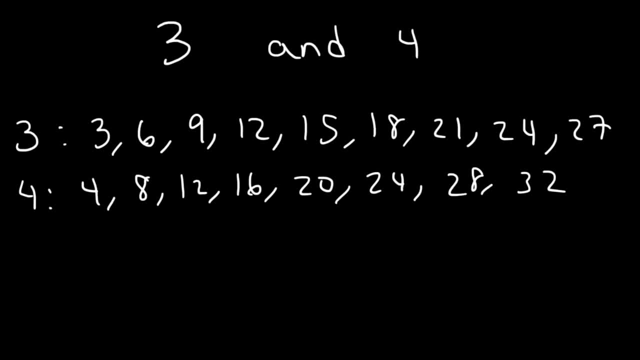 So now, which ones are common multiples of 3 and 4?? 12 is a common multiple between 3 and 4.. As we can see, it's found in both lists, And another multiple is 24.. Now, which of these is the least common multiple? Well, 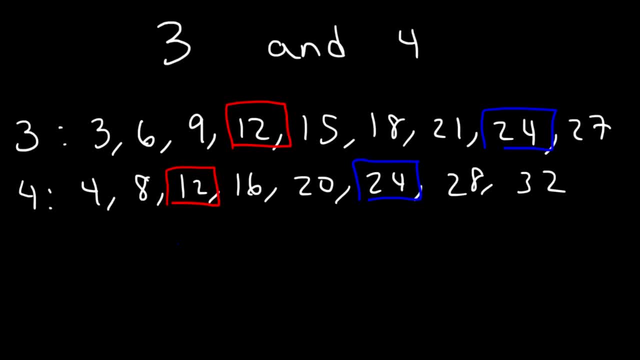 12 is lower than 24, so 12 is the LCM. It's the least common multiple between 3 and 4.. Now let's work on another example. What is the least common multiple between 6 and 9?? Feel free to pause the video and. 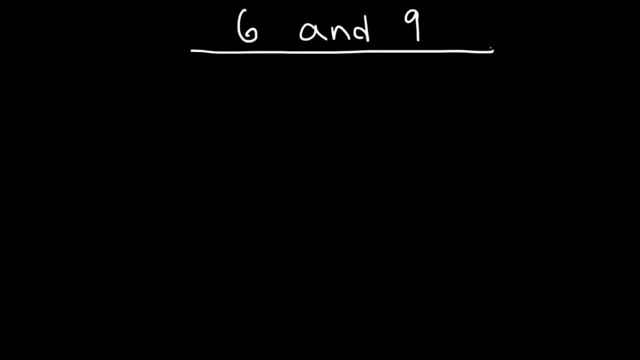 work on this example, go ahead and try. so let's make a list. let's start with 6, so we have 6, 12, 12 plus 6 is 18, 18 plus 6 is 24, and then it's going to be 30, 36, 42 and so forth. 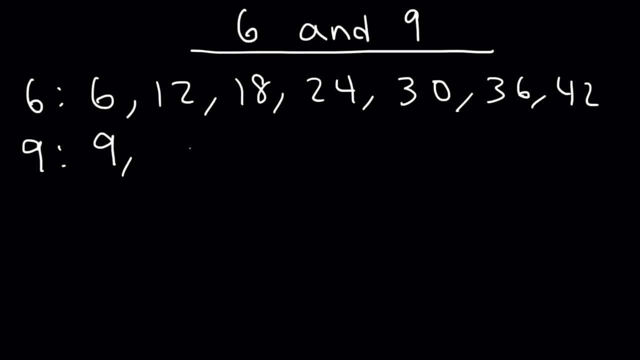 now let's do the same with 9. we're going to have 9, 18, 27, 36, 45, 54 and so forth. so 18 is a common multiple between 6 and 9 and also 36, but the least common multiple. 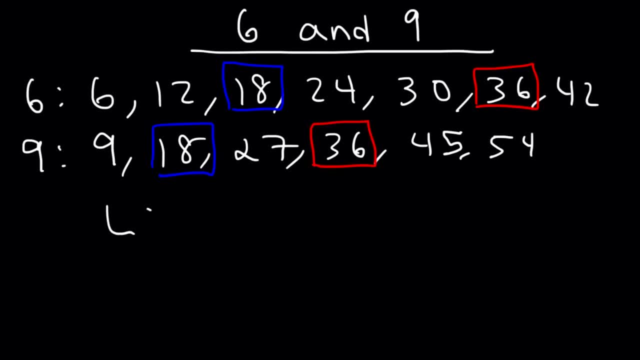 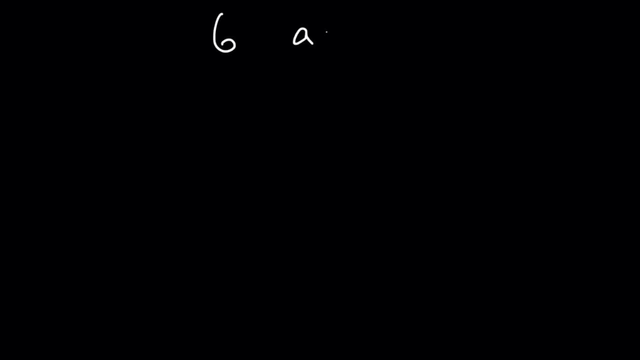 is 18. it's the lowest of the two numbers, so that's going to be the LCM. in this example it's 18. now how can we get the same answer using prime factorization? factors of 6 are 3 and 2. factors of 9 are 3 and 3. 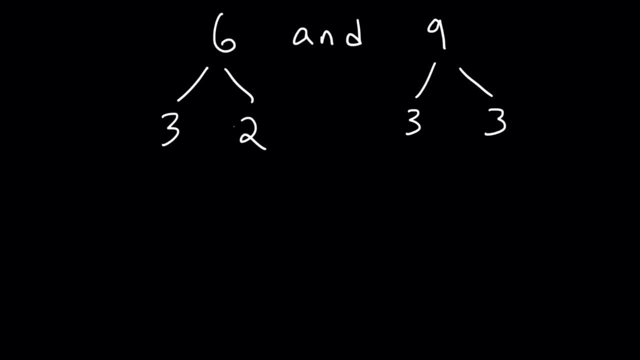 so both numbers. well, only 6 contains the 2, but in our least common multiple it has to have at least one 2. now what about 3's? how many 3's should we use? should we use 1, 3? should we use 2, 3's or all 3? 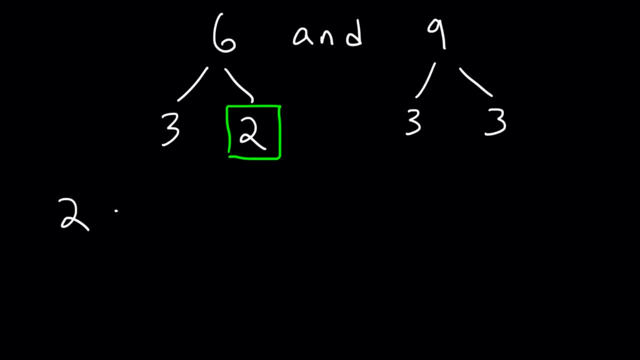 you want to use the most number of 3's. you want to use the most number of 3's. you want to use the most number of 3's that's found in one particular number. In this example, we use the most number of. 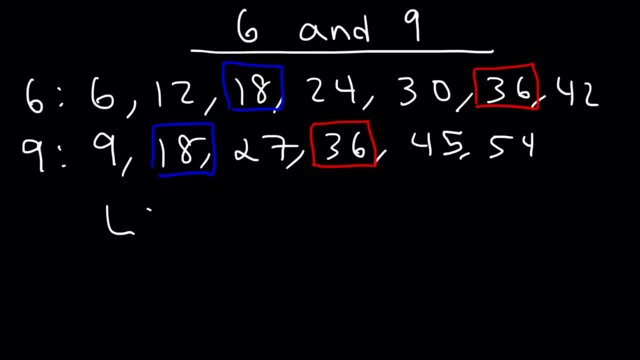 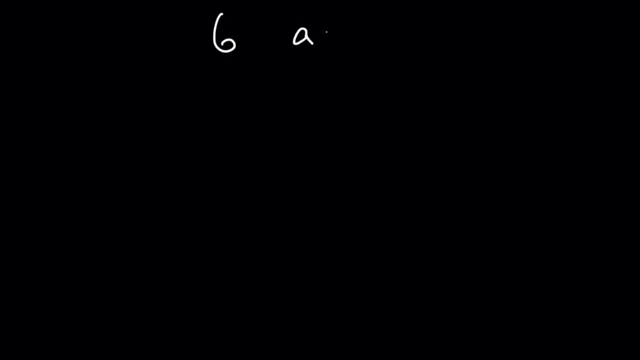 is 18. it's the lowest of the two numbers, so that's going to be the LCM. in this example it's 18. now how can we get the same answer using prime factorization? factors of 6 are 3 and 2. factors of 9 are 3 and 3. 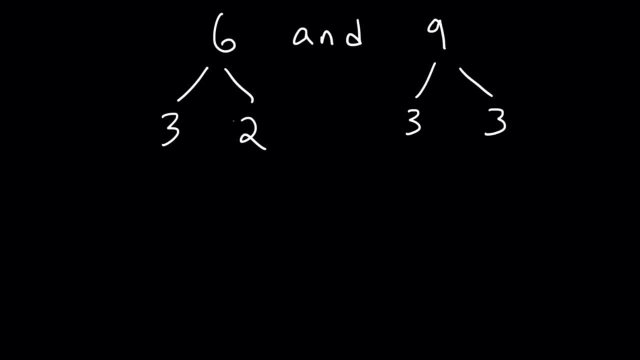 so both numbers. well, only 6 contains the 2, but in our least common multiple it has to have at least 1- 2. now what about 3's? how many 3's should we use? should we use 1, 3? should we use 2, 3's or all 3? 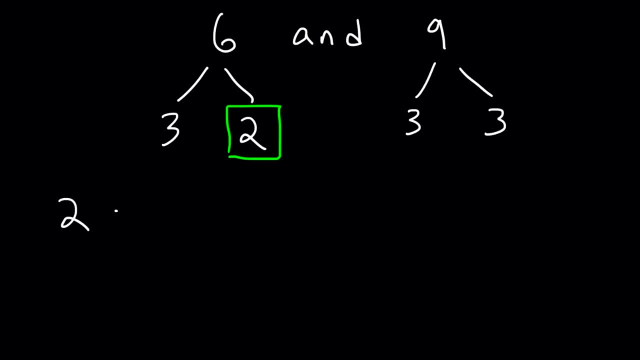 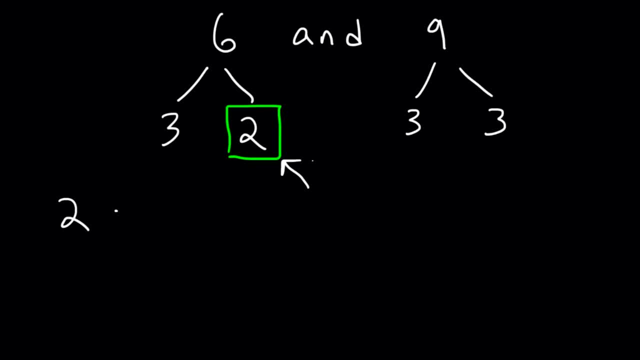 number of twos that's found in one of the numbers, which is just six. the most number of threes that's found in one number is two- threes. so that's what you want to do: we need to use two threes. three times three is nine. two times nine. 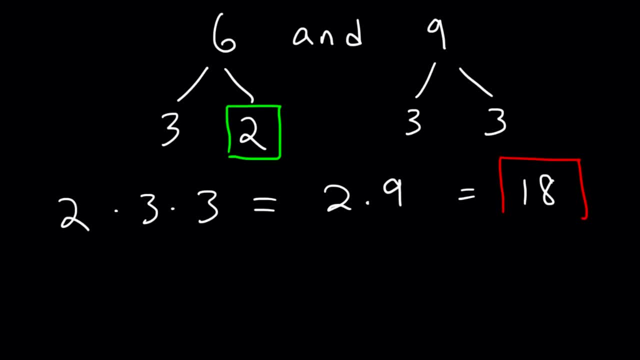 is eighteen. as you can see, it gives us the LCM, the least common multiple. now let's move on to our next example. try this one: 24 and 32, so build a list and also use prime factorization to get the same answer. factors of 24 are six and 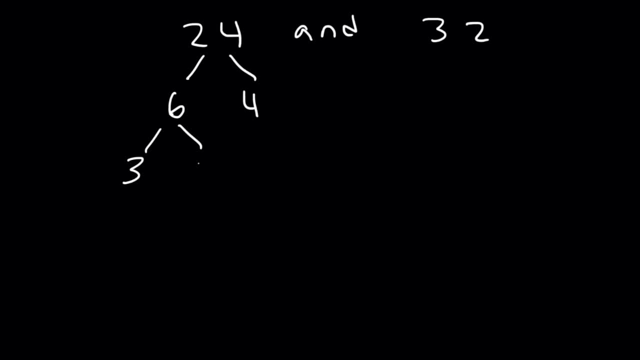 four. factors of six are three and two, factors of four are two and two, factors of 38 are eight and four and factors of eight are four and two, and four is going to be two and two. so the prime factors, as you can see, are 3, 2, 2. 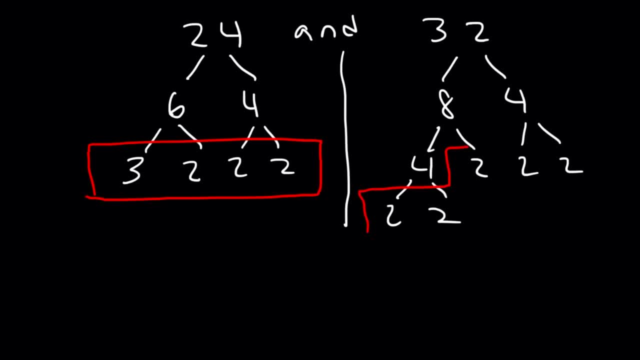 and 2 for 24 and for 32. it's the five twos that we see here. so how many threes should we use to find the LCM? the most number of threes that are found in any one of these two numbers is there's only one three, so we're just going to use 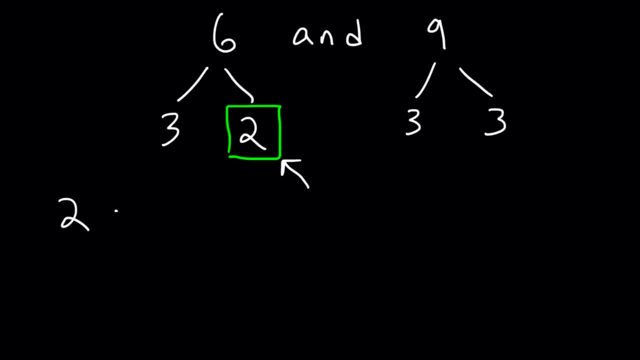 twos that's found in one of the numbers, which is just six. The most number of threes that's found in one number is two- threes. so that's what we want to do: We need to use two, threes Three times three is nine. two times nine is eighteen, As you. 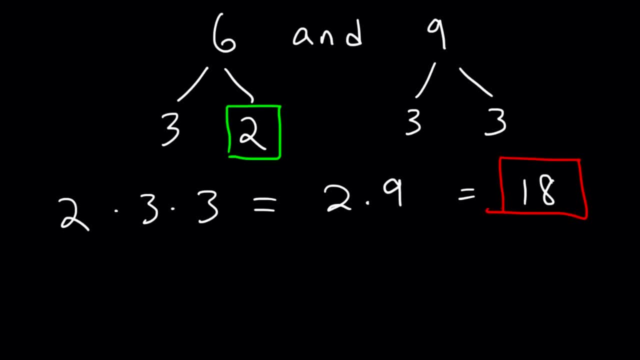 can see, it gives us the LCM, the least common multiple. Now let's move on to our next example. Try this one: 24 and 32.. So build a list and also use prime factorization to get the same answer. Factors of 24 are 6 and 4.. 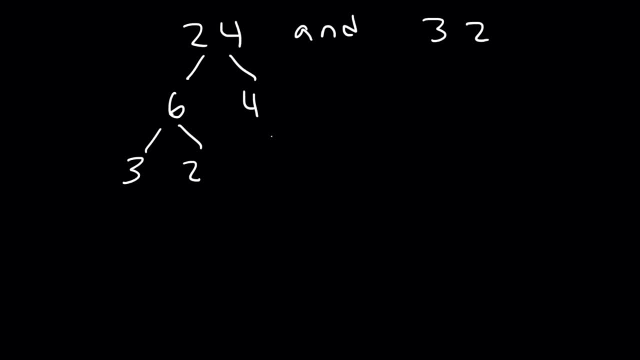 Factors of 6 are 3 and 2.. Factors of 4 are 2 and 2.. Factors of 38 are 8 and 4, and factors of 8 are 4 and 2, and factors of 2 and 3 are 8 and 4.. 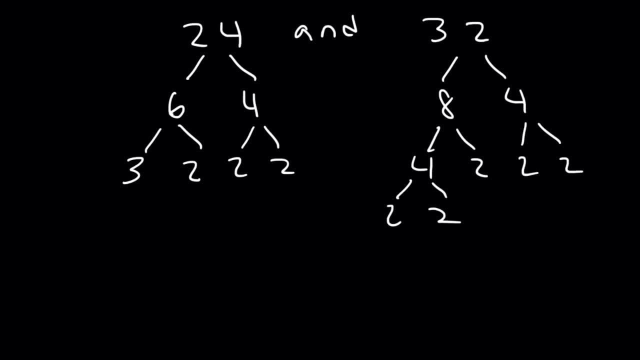 And 4 is going to be 2 and 2.. So the prime factors, as we can see, are 3, 2,, 2, and 2 for 24.. And for 32, it's the 5- 2's that we see here. 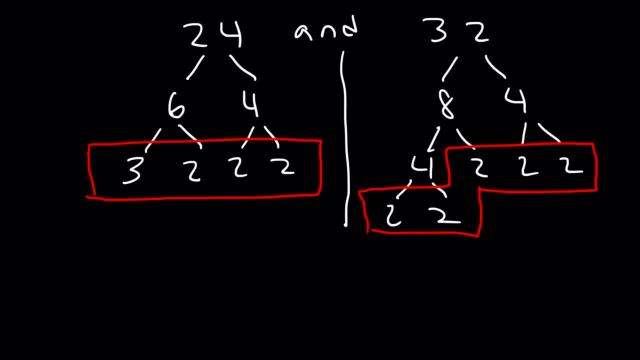 So how many 3's should we use to find the LCM? The most number of 3's that are found in any one of these 2 numbers is there's only one, 3.. So we're just going to use that for the prime factorization. 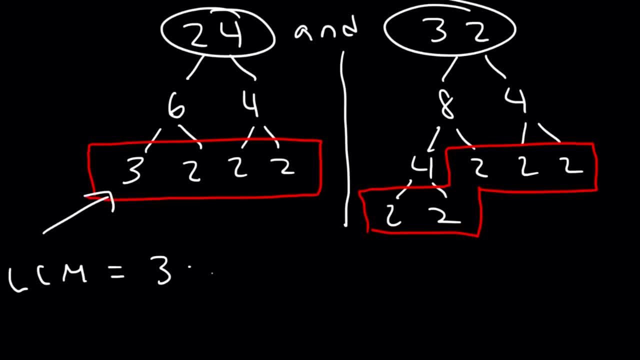 Now, what is the most number of 2's that's found in one single number? On the left side, we have 3- 2's. On the right side, we have 5- 2's. So we're going to have to use 5- 2's. 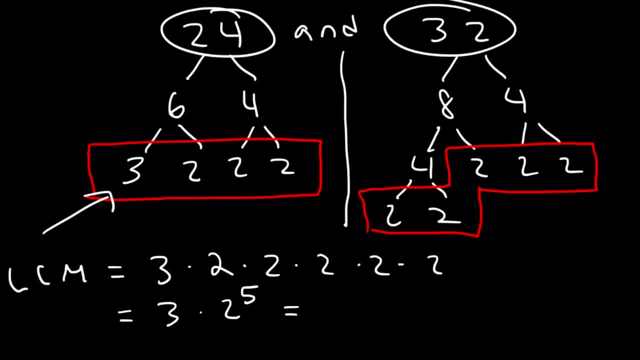 5: 2's is basically 2 to the 5th power. It means you're multiplying 2, 5 times And 2 to the 5th power. we know it's 32 because that's where we got it from. 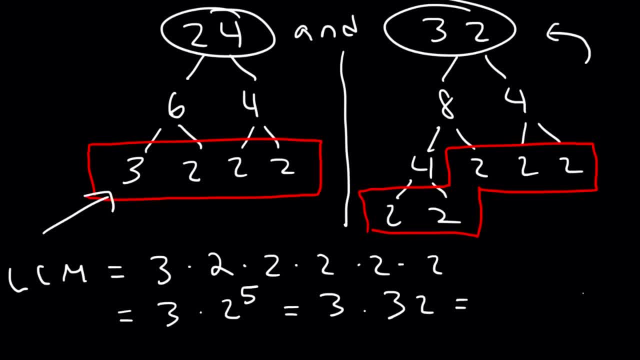 So it's 3 times 32.. 3 times 30 is 90.. 3 times 2 is 6.. 90 plus 6, that's going to be 96.. So that's the LCM between the 2 numbers. 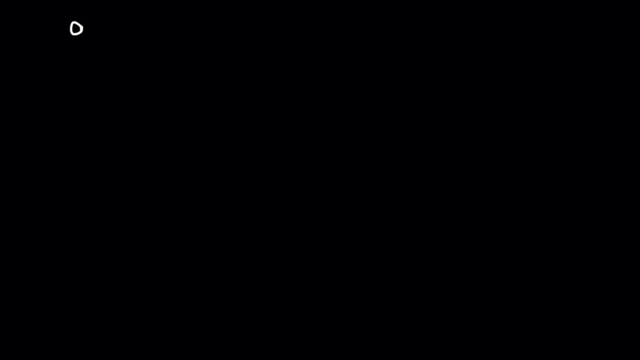 Now let's prove it by making a list. Also, you can also divide. 96 divided by 24 has to give us a whole number if 96 is a multiple of 24.. When you divide these 2, you should get 4.. 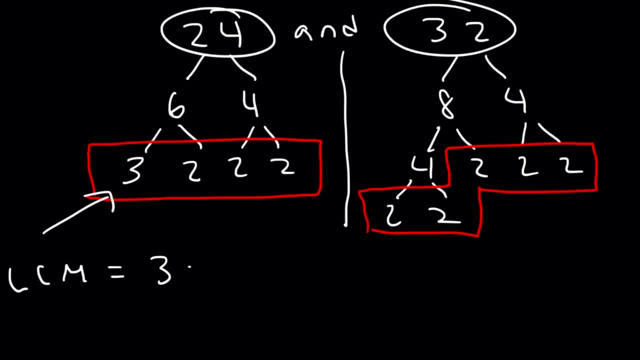 that for the prime factorization. now, what is the most number of twos that's found in one single number. on the left side, we have three twos. on the right side, we have five twos. so we're going to have to use five twos. five twos is. 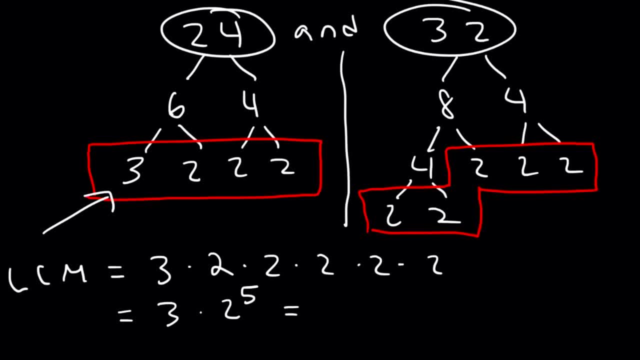 basically two to the fifth power. it means you're multiplying two five times and two to the fifth power. we know it's 32 because that's where we got it from. so it's three times 32. three times 30 is 93 times 26. 90 plus six that's going to be 96. so that's the. 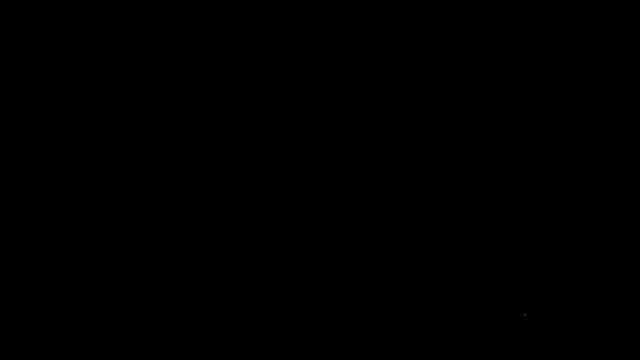 LCM between the two numbers. now let's prove it by making a list. also, you can also divide. 96 divided by 24 has to give us a whole number. if 96 is multiple 24, when you divide these two you should get four: 96 divided by 24. 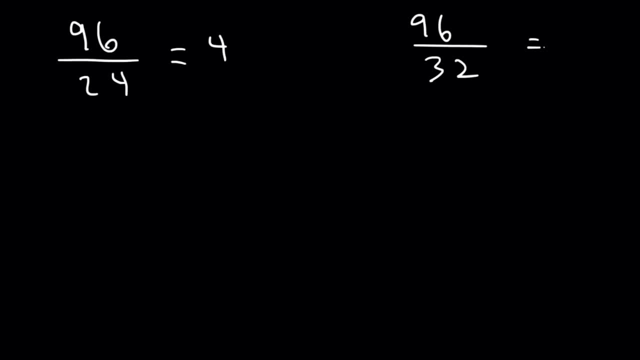 I mean 32. the other number is three. so that tells us that 96 is a common multiple between 24 and 32, because when you divide it by both of these numbers you get a whole number. now let's make a list. so multiples of 24 are itself 48, 72. 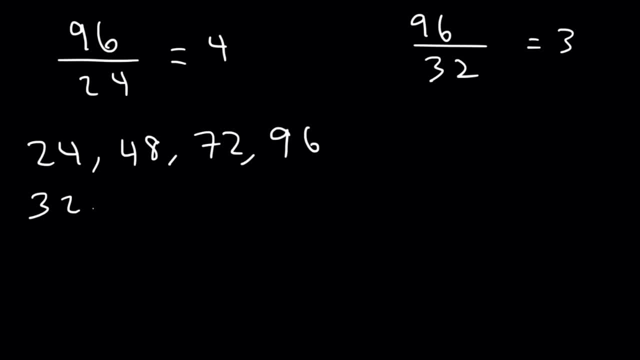 and 96. multiples of 32 are 32, 64 and 96. if you keep adding 32, as you can see, I 96 is indeed the LCM between 24 and 32. now what is the least common multiple between 12, 15 and 20? so pause the video and work on that example. go ahead and. 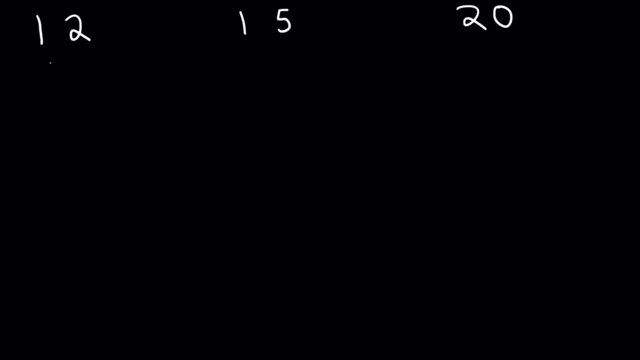 take a minute. common factors of 12 are four and three, and we could break down four into two and two. so therefore, this is the prime factorization: 2, 2 & 3. factors of 15 are 5 & 3 and factors of 20 are 5 & 4 & 4. we could break that into two and two. so these are the the 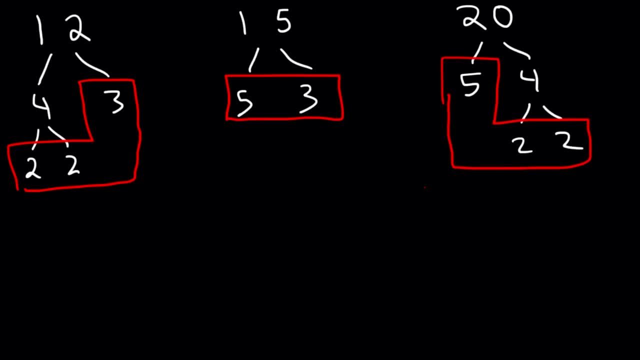 prime factorization of these numbers. so now, what is the LCM? so how many twos should we use? 해 number of twos in 12 are two twos, There's 9 in 15, and the most number of twos in 20 is. 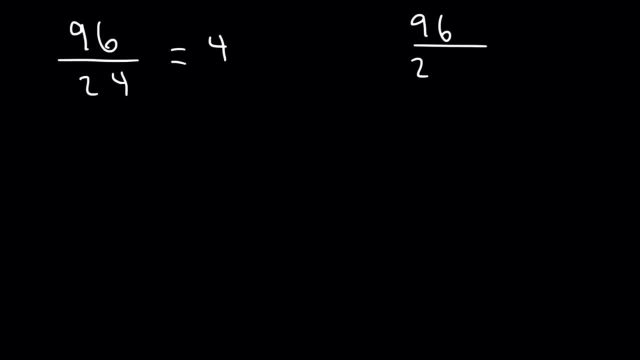 96 divided by I mean 32,. the other number is 3.. So that tells us that 96 is a common multiple between 24 and 32.. Because when you divide it by both of these numbers you get a whole number. 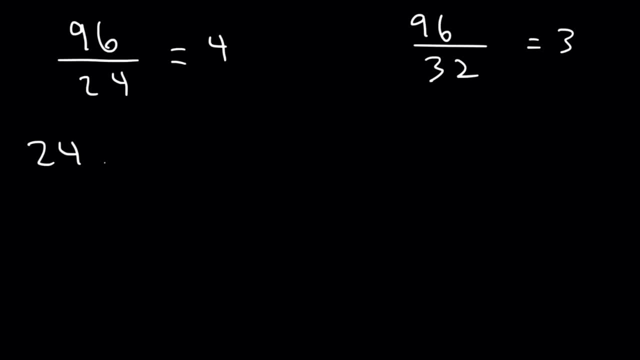 Now let's make a list. So multiples of 24 are itself 48,, 72, and 96.. Multiples of 32 are 32,, 64, and 96, if you keep adding 32.. As you can see, 96 is indeed the LCM between 24 and 32.. 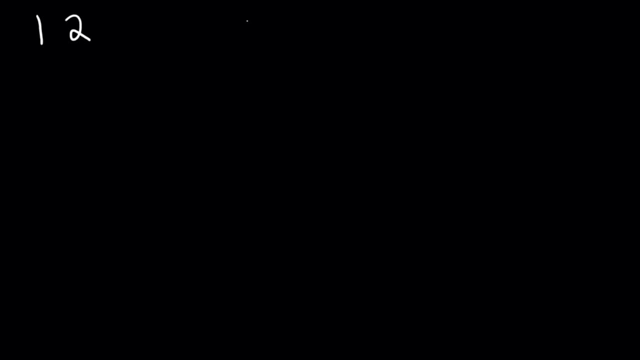 Now what is the least common multiple between 12,, 15, and 20?? So pause the video and work on that example. Go ahead and take a minute. Common factors of 12 are 4 and 3.. And we can break down 4 into 2 and 2.. 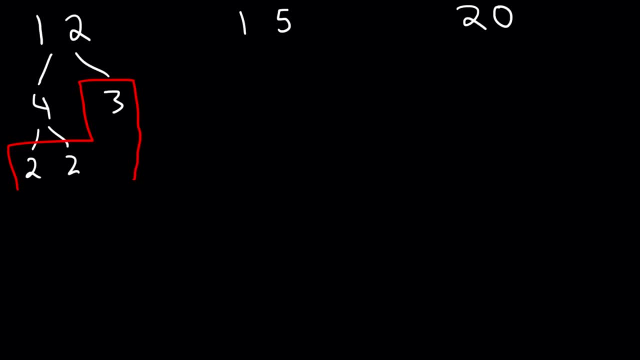 So therefore, this is the prime factorization: 2,, 2, and 3.. Factors of 15 are 5 and 3.. And factors of 20 are 5 and 4.. And 4, we can break that into 2 and 2.. 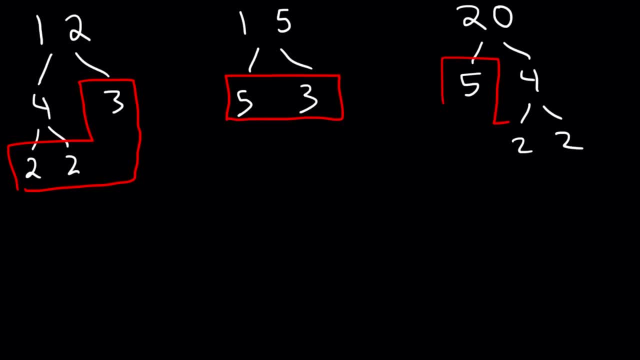 So these are the prime factorization of these numbers. So now, what is the LCM? So how many 2s should we use? The most number of 2s in 12 are 2 2s. There's none in 15, and the most number of 2s in 20 is 2 2s. 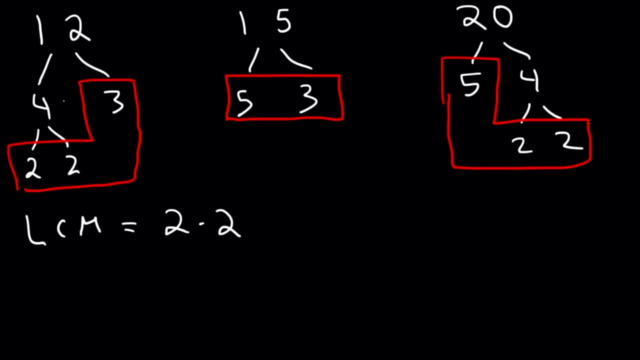 So we're going to use 2, 2s. The most number of 3s in any number is simply 1, 3.. And the most number of 5s we have 1, 5 here and 1, 5 here. 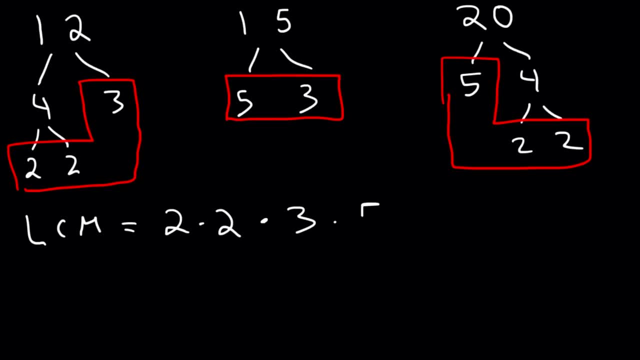 So we're just going to use only 1, 5.. 2 times 2 is 4.. 3 times 5 is 15.. And 4 times 15 is 60. So, therefore, the LCM is 60.. 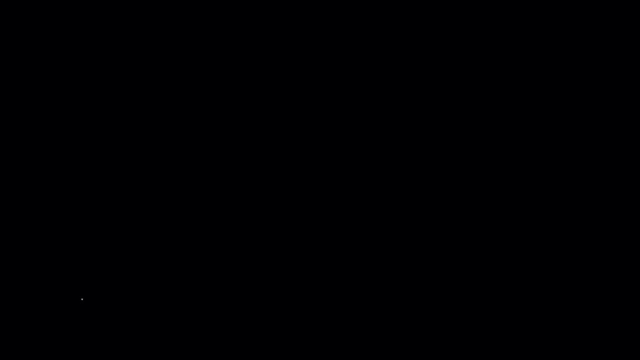 So each number- 60- should be divisible by each number. If we divide 60 by 12,, it gives us 5.. 60 divided by 15 is 4. And 60 divided by 20 is 3.. So 60 is a common multiple between 12,, 15, and 20, based on what we can see. 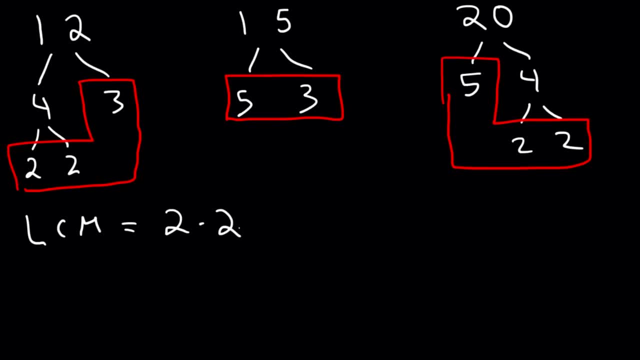 two twos. So we're going to use two twos. The most number of threes in any number is simply one three And the most number five. so we have one five here and one five here, So we're just going to use only one five. 2 times 2 is 4, 3 times 5. 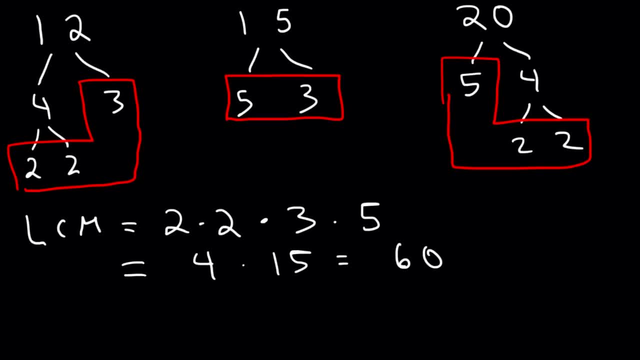 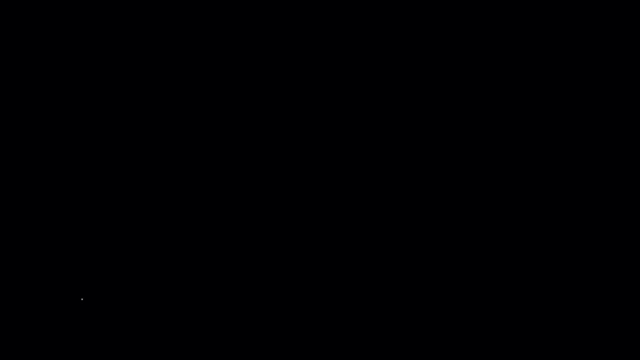 is 15, and 4 times 15 is 60. So therefore, the LCM is 60. So each number- 60- should be divisible by each number. If we divide 60 by 12, it gives us 5. 60 divided by 15. 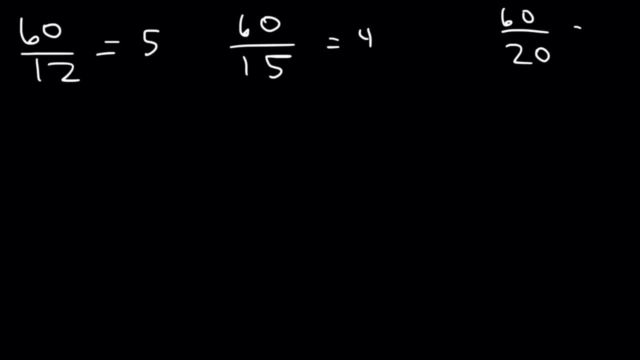 is 4, and 60 divided by 20 is 3.. So 60 is a common multiple between 12,, 15, and 20, based on what we can see. Now, let's see what we can do. Now, let's see what we can do. 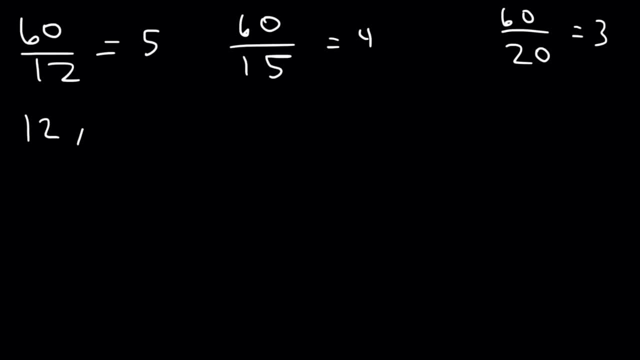 Now let's make a list. Multiples of 12 are 12,, 24,, 36,, 48, and 60. Multiples of 15 are 15,, 30,, 45, 60. And for 20, it's itself 40 and 60. So we can clearly see that 60 is. 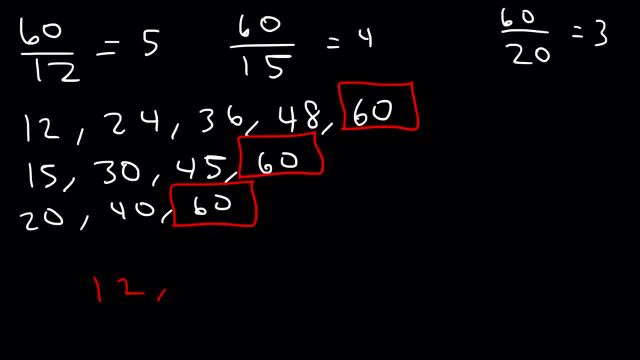 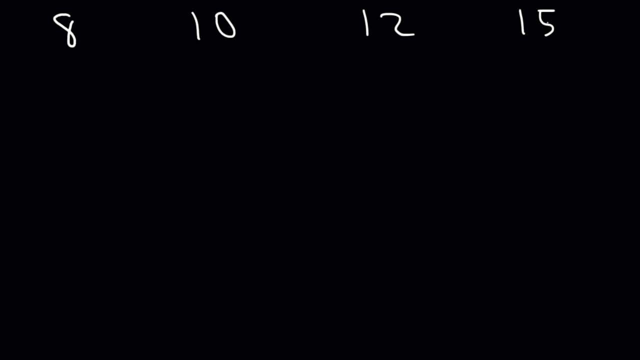 indeed the LCM between 12,, 15, and 20.. So 60 is the answer. Let's try an example with four numbers: 8,, 10,, 12, and 15.. So try that. Pause the video. 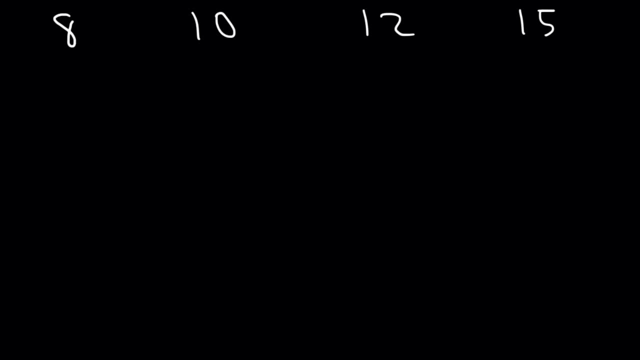 and work on that example And then unpause it to see the solution. So let's start with 8.. We can break it down into 4 times 2.. And 4 is 2 times 2.. So the prime factorization. 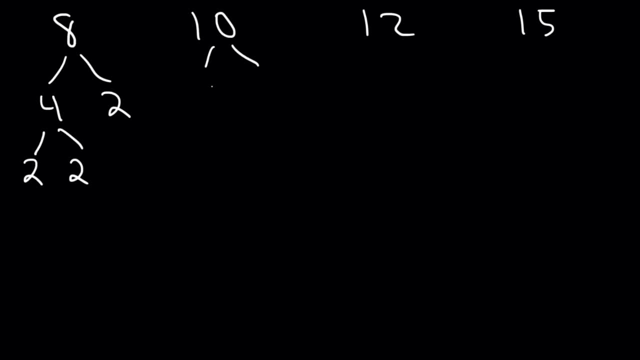 of 8 is 2 times 2 times 2.. 5, I mean 10,, not 5.. 10 is 5 times 2. And 12 is 4 times 3. And 4 is 2 times 2.. 15, we. 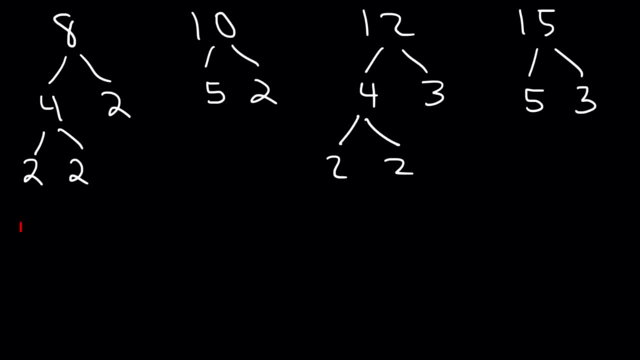 can break it into 5 and 3.. So now let's go ahead and find the LCM. So what is the most number of 2s that you see in any given number? So 8 contains 3, 2s. That's the most number of 2s. 10 only has one, 2.. 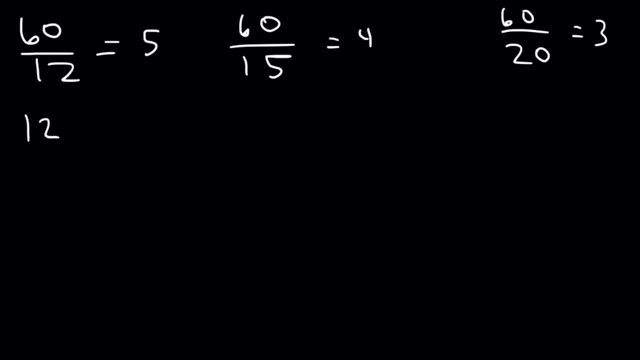 Now let's make a list. Multiples of 12 are 12,, 24,, 36,, 48, and 60.. Multiples of 15 are 15,, 30,, 45, 60. And for 20, it's itself 40 and 60. 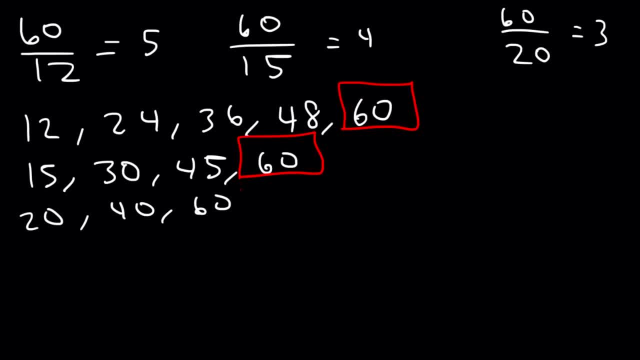 So we can clearly see that 60 is indeed the LCM between 12,, 15, and 20.. So 60 is the answer. Let's try an example With four numbers: 8,, 10,, 12, and 15.. 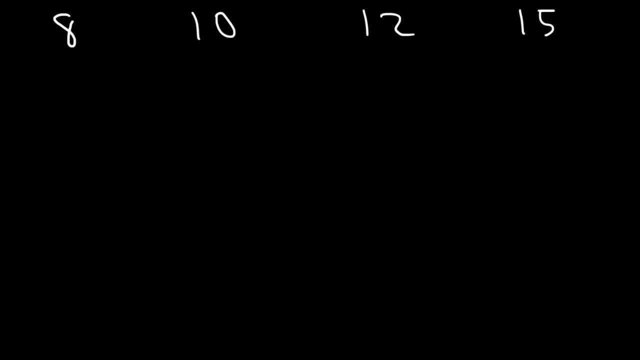 So try that: Pause the video and work on that example And then unpause it to see the solution. So let's start with 8.. We could break it down into 4 times 2.. And 4 is 2 times 2.. 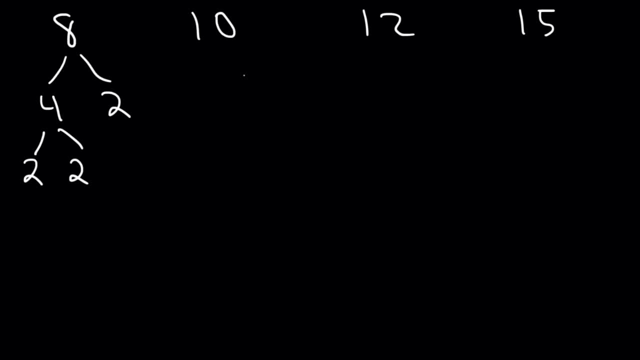 So the prime factorization of 8 is 2 times 2 times 2.. 5, I mean 10., Not 5. 10 is 5 times 2.. And 12 is 4 times 3.. And 4 is 2 times 2.. 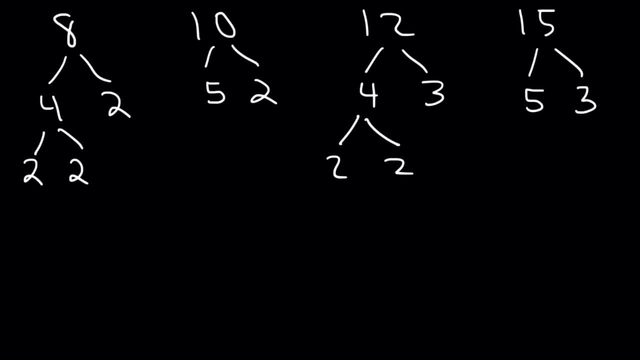 15,. we could break it into 5 and 3.. So now let's go ahead and find the LCM. So what is the most number of 2s that you see in any given number? So 8 contains 3 2s. 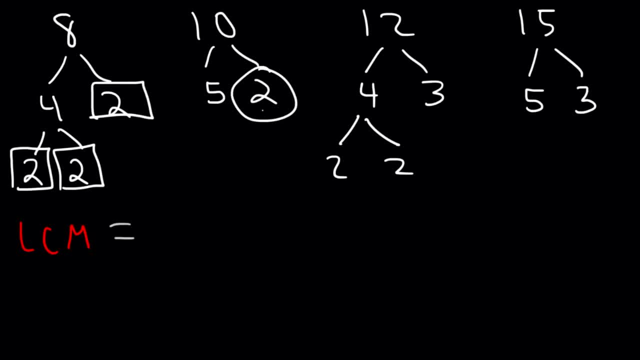 That's the most number of 2s. 10 only has 1 2. And 12 has 2 2s. So the most number of 2s in any number is 3 2s. Now let's move on to 3.. 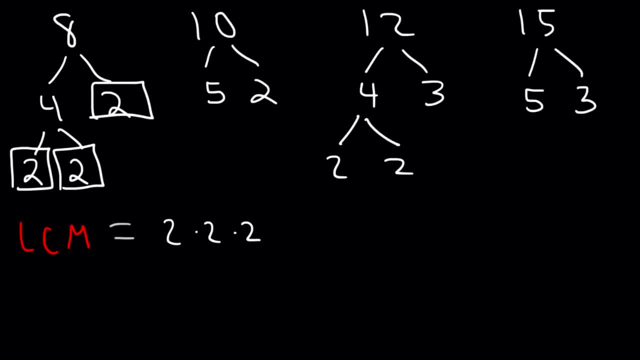 What's the most number of 3s in any given number? 12 has 1, 3.. 15 has 1, 3.. So the most number of 3s is just 1, 3.. What about the most number of 5s? 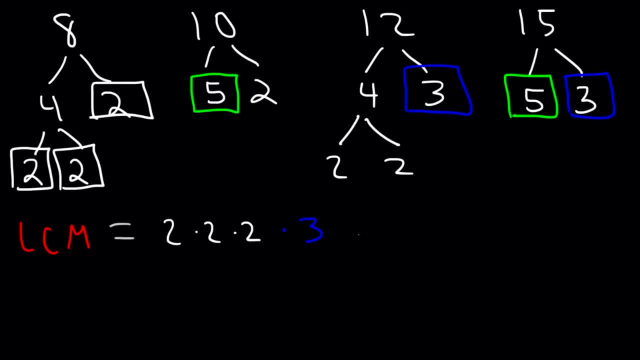 10 has 1, 5.. 15 has 1, 5. So we only need 1, 5.. Now we know that 2 times 2 times 2 is 8.. 3 times 5. 5 is 15.. 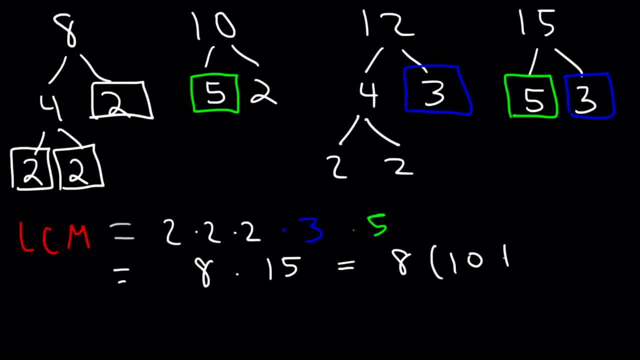 So 8 times 15 is the same as 8 times 10 plus 5.. 8 times 10 is 80.. 8 times 5 is 40.. And 80 plus 40 is 120.. So 8 times 15 is 120..